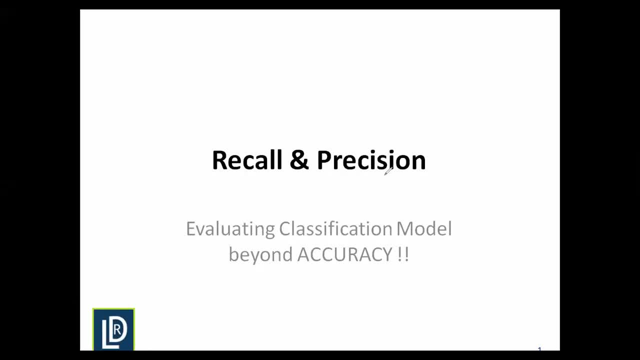 Hello and welcome to this session on recall and precision. Both of them are nothing but evaluation metrics which help us identify how good a classification model is. Now a lot of people wonder: why is there a need of any other evaluation metric when we have accuracy, which is so intuitive and so simple to understand? So in today's session we'll try to. 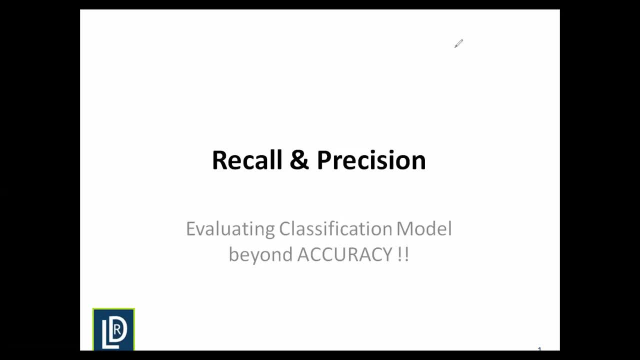 understand the precise need of both these evaluation metrics, and we'll try to understand the need of both these evaluation metrics. So in today's session, we'll try to understand the precise need of both these evaluation metrics, try to do this using a live case study. Now, before we go there, I want to make 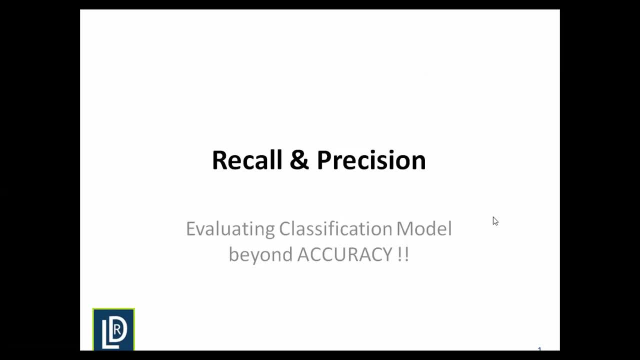 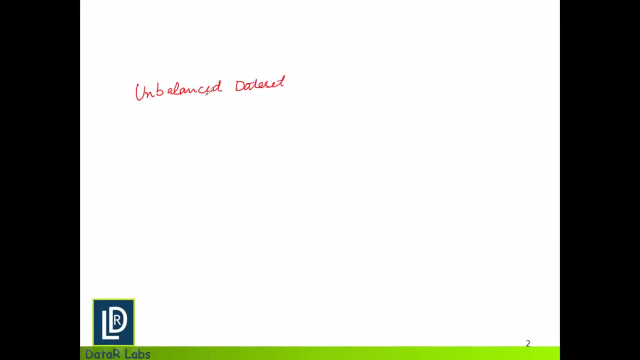 sure that we know one thing which is very important, especially in this case of recall and precision. So, for those who have not heard anything like unbalanced data set, unbalanced data set- it's your time to understand more about it. Now, what is unbalanced data set? 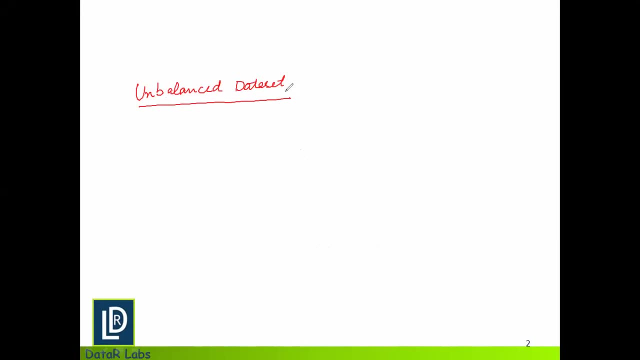 So unbalanced data set is a data set where the target variable or the y variable has disproportionate levels in that. Now, what do I mean by that? So let's say I have this data set and I'm talking about a binary data set, where my target variable has just two levels, either a one 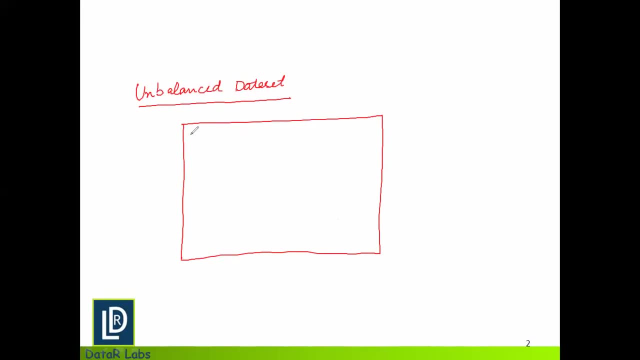 or zero. So let's say we have this data set with few independent or predictor variables- let's say four of them- and then we have a target variable which is y. So these are predictor variables and this is a target variable. So what I mean by unbalanced data set is: so let's assume this data set is about credit risk. 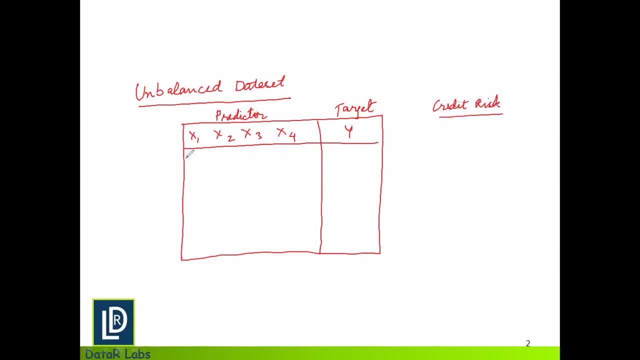 So, given the characteristics of a person who is coming to take a loan from the bank- let's say: x1 is age, x2 is income, x3 is the amount of loan, x4 is probably the purpose of the loan- will have whether that person would default or whether that person will not default. 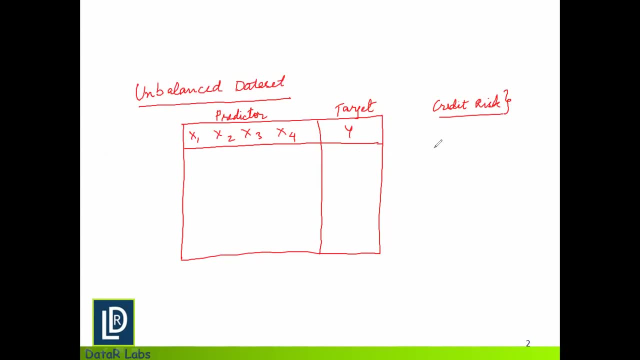 So in a typical situation of credit risk modeling, people who are defaulting are far lesser than people who are not defaulting. So if one corresponds to people who are defaulting, people who are defaulting and zero corresponds to people who are repaying the loan back. 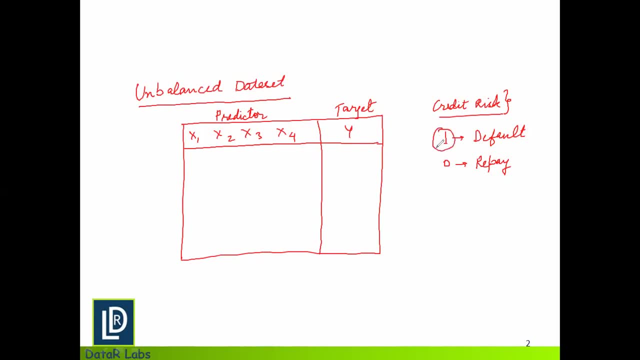 number of ones. number of ones are far lesser than number of zeros, which means that in this data set I would have far lesser ones than the number of zeros. So this is what unbalanced data set is. On the contrary, a balanced data set would be. 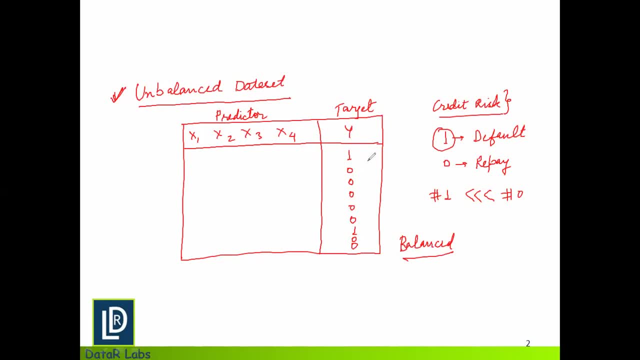 a balanced data set would be when I have an equal proportions for both one and zero, or at least very close to equal proportion. So I would have 50 percent of ones and I'll have 50 percent of zeros, So very close by to each other. 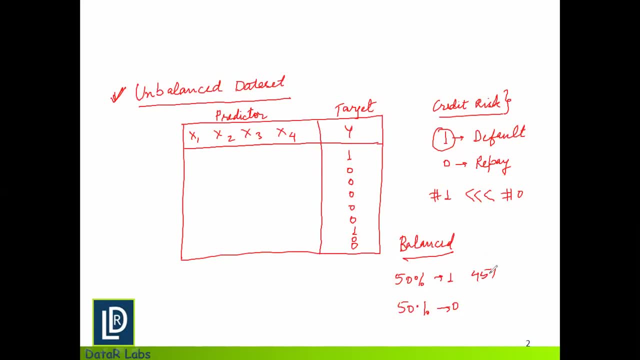 or maybe this can go on to 44,, 45 and this can be 55. Still, they're very close to being called as balanced data set as opposed to unbalanced data set, where, in a typical case of credit risk, I'll have around 90-95 percent of people who are repaying the loan back. So I'll have around 99.5 percent. 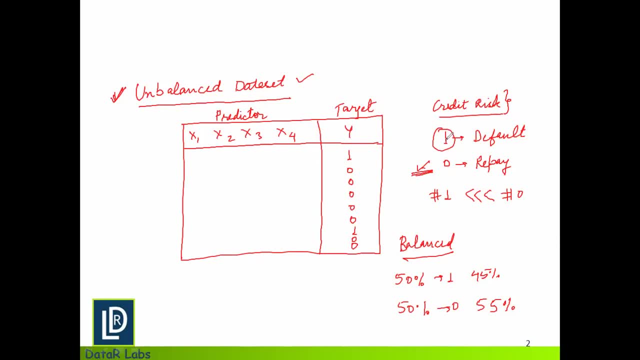 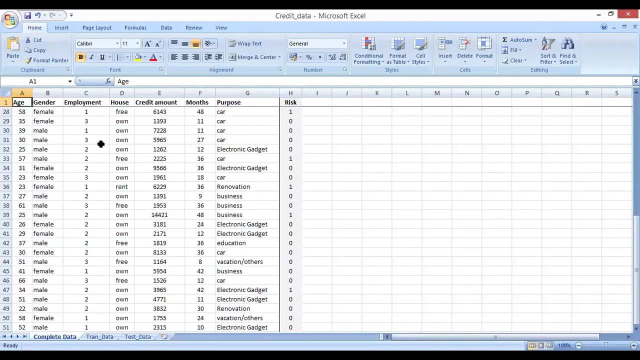 of zeros and I'll just have around five to ten percent of ones in the data set. So this is highly unbalanced data set. Now let's get to the example. Let's start with a single example and try to understand precision and recall with this understanding of unbalanced data set. 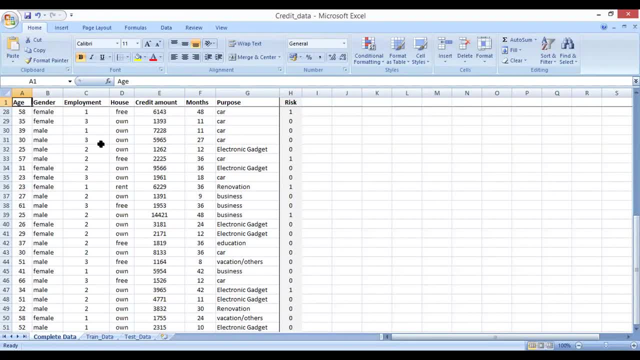 So here's the data, the same data which we were talking about credit risk scoring. So, given these, which are age, gender, employment, type of employment, house, again, the type of housing in which that person is living, whether it's a free accommodation, whether it's a owned house, whether it's a rented house- and then the amount, of next variable is the. 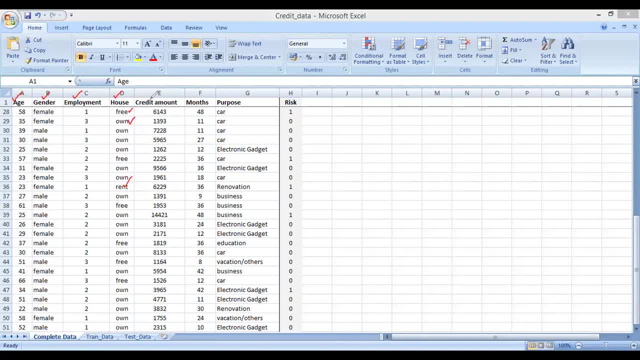 credit amount: the amount of credit which has been taken from the bank, for the duration the loan has been taken and for what purpose the loan has been taken. these are all my x variables. so i have seven x variables, from x1 till x7, and then this is a y variable or a target variable. so for 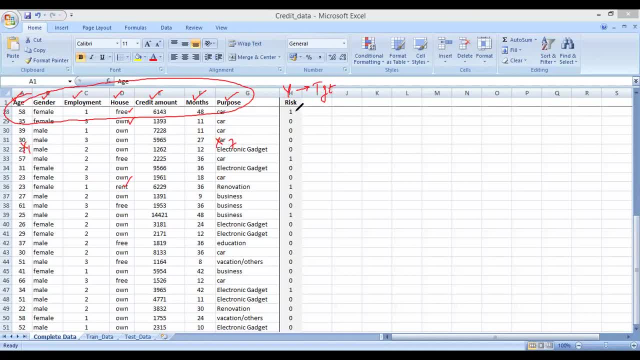 every characteristic, i would have risk involved. so, for example, if a person is 30 years of age, she's a female, this is the employment category- and she owns the house. there's the amount of credit she has taken, and for 36 months- and this was a car loan- this lady repays back and thereby we have entered a zero against. 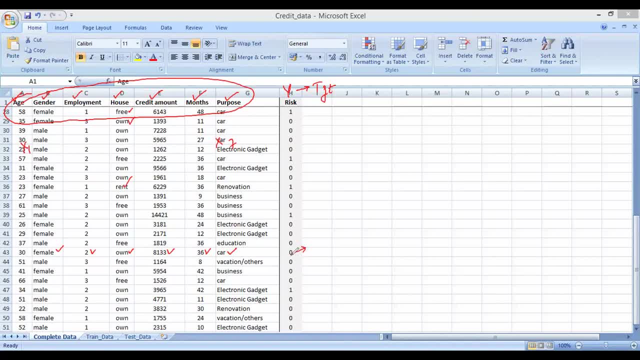 her name or against her characteristics. if i take another example from this row, number 36, i see that for all these characteristics, with all these characteristics, this lady has defaulted, and thereby i get a one now. the typical behavior of this data set is the typical behavior of this data. 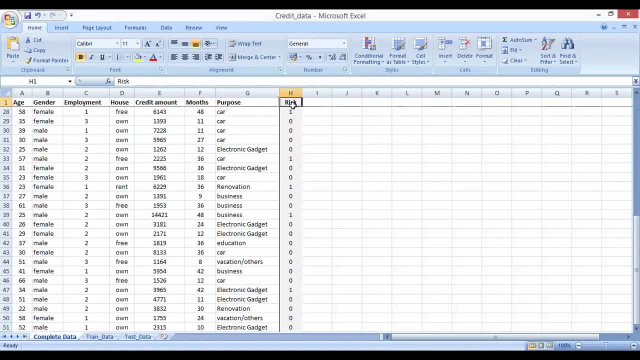 set is that i get far more ones than the number of zeros. so if i take the total number of row items, i have 50 row numbers, out of which i just have eight defaulters, which means the proportion of my data set is number of ones is 16 percent. 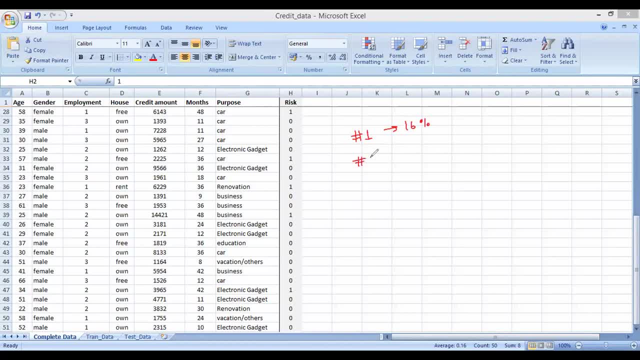 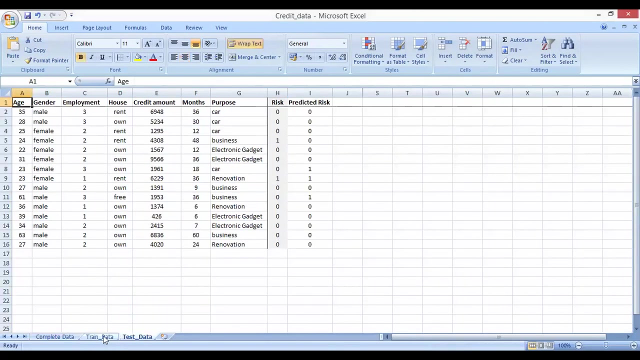 whereas number of people who are repaying back- so number of zeros- is 84 percent. highly unbalanced data set. now, with these data sets, we need to advance to other evaluation metrics like recall and precision, so we'll exactly see how this works. now this data set has been divided into train set and test set. train set is 70 percent of the complete. 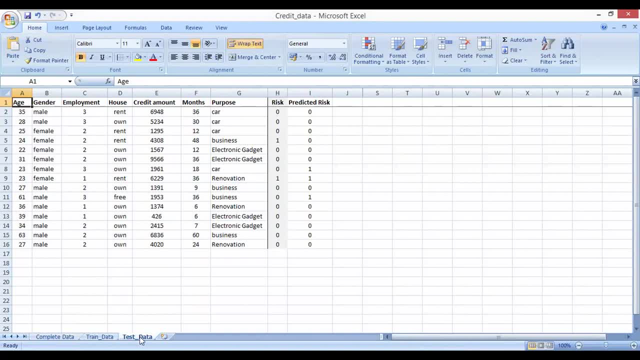 data set and test set is 30 percent of the complete data set using train set. i have made the model already and using that model i have done a prediction with. the resultant of that prediction is there in this column i, which has been annotated as predicted risk. 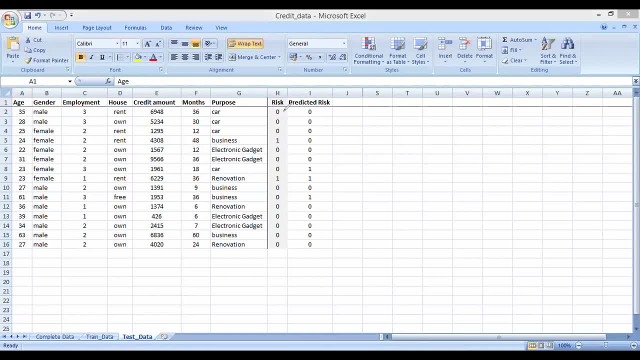 so now, for every row in the test set, i have the actual risk and i have a predicted risk. so, for example, these top three rows have been predicted perfectly by my model, whereas this row has been incorrectly predicted, and so on. now for this y and y cap, i have 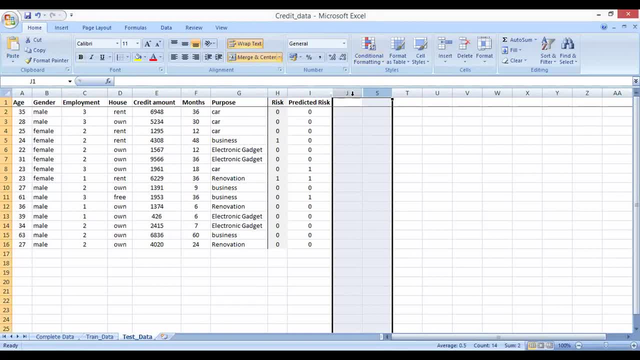 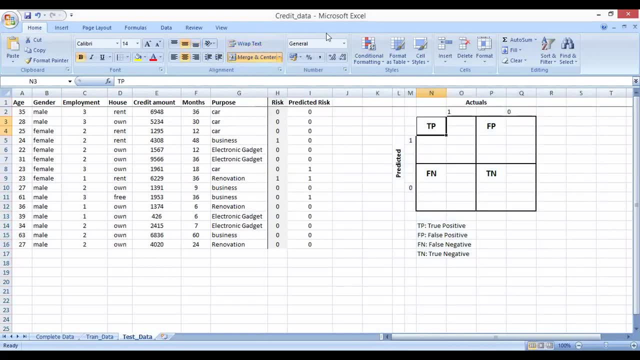 a confusion matrix. now, if i count these, why do what you'll see here? and these two rows are true or false. this is the information SAS can project in through the analysis here. so, for example, if cells appear in hyperbolic values, then there happened a doubt. if they are true or false, and whose or false 누 is the query case value than that means in the values case after context element here we insert, which is 2.aries, 1. nikov, 1.14 and next Das quote, that is, ili 1.41-10.1 is 0 and 0 as a corrector of the 1-true an. 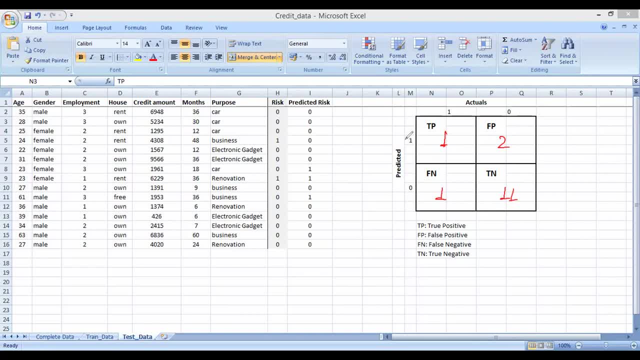 how to make confusion matrix. they can probably go back and check my other session as to how do we calculate or design this confusion matrix. Now, moving on, with this kind of a confusion matrix, the accuracy, what I get is nothing but 1 plus 11 over 15, which is 80 percent. 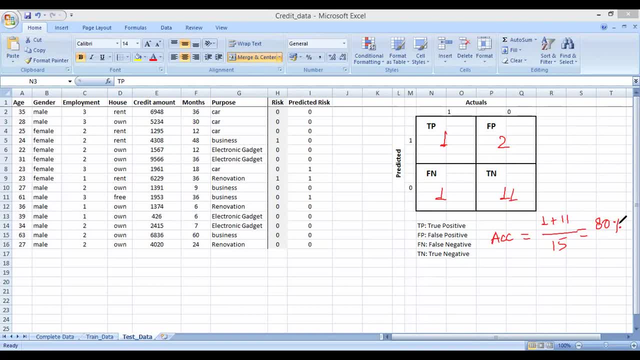 absolutely fantastic accuracy, isn't it? accuracy of 80 percent means my model is doing really good, but I'll give you a very dirty trick to bump up this accuracy instead of this model which is predicting these values. for my risk, what I'll go on to do is I would probably make a very simple model and I would just enter all zeros. 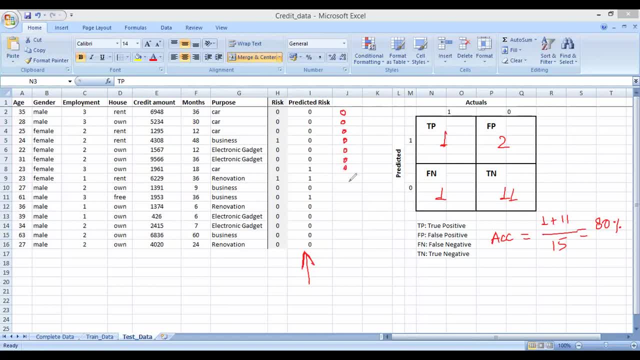 so I would just enter all zeros instead of making this model. so if I do this, so let's say this is my model one and this is my model two, where I am predicting everyone to be a non-defaulter and thereby I'm giving loan to everyone. 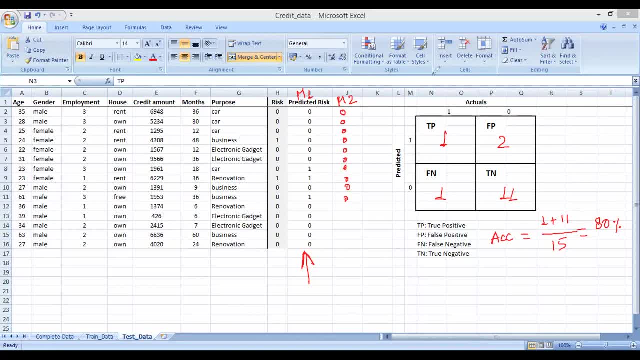 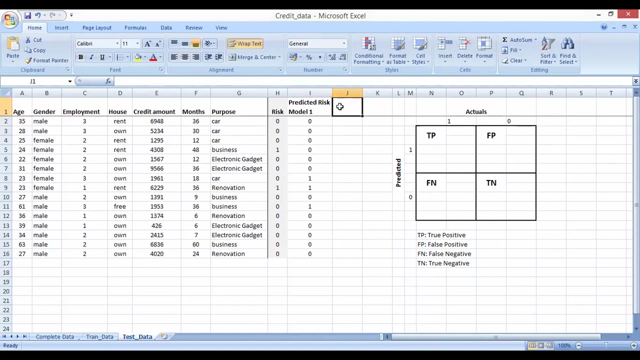 so this is my second strategy to model. my first strategy is: so let's kind of write this down in this sheet. so this is my model one, this is my model one, and let's say this is my model two, where I am predicting everyone to be a non-defaulter. 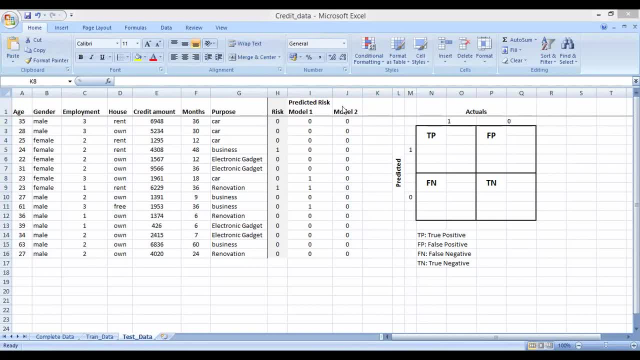 now, what would be my new confusion matrix? according to this new model, my new confusion matrix would be: my true positives would be zero, my false positives would be zero, my false negatives would be two and my true negatives would be 13.. and now, if I calculate the 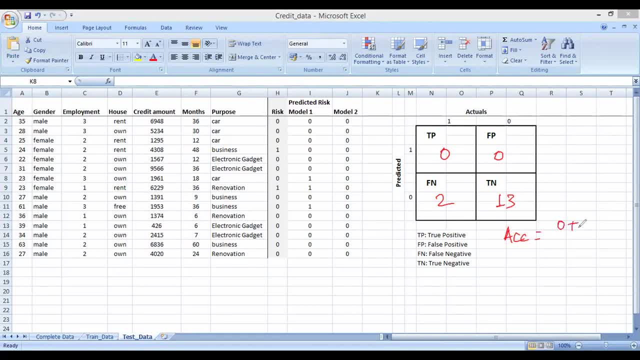 accuracy: it is zero plus 13 over 15.. fantastic, with a little dirty trick and a much simpler model, I'm getting much better accuracy, isn't it? but let's kind of just review what we have done here. so what we did was we, with model one, we were getting an accuracy of 80 percent, but with model two, we were getting an. 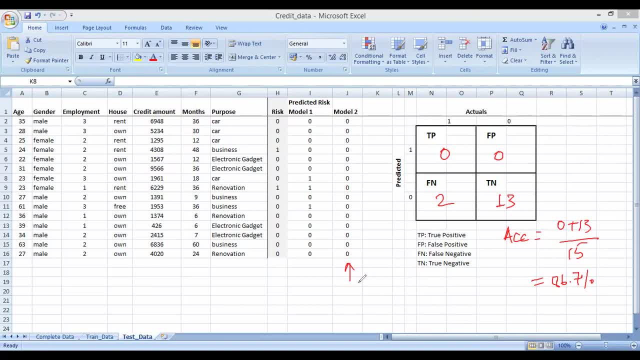 accuracy of 86.7 percent, almost 87 percent now from business perspective. we are not making any effort to identify defaulters, which means the strategy is bad, because Part of the problem is that the strategy is bad because the whole concept behind loan industry is they want to correctly and as accurately as possible, want to identify. 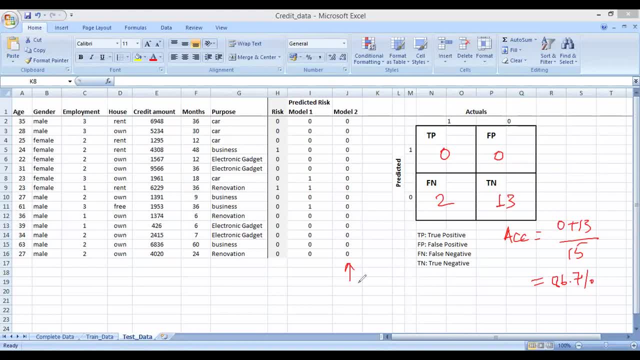 the people who might default on me, and thereby I want, or I don't want, to give loans to these people. so this turns out to be a bad strategy from business point. but my accuracy somehow increased, so this looks like a big contradiction between business and reality: business, reality and 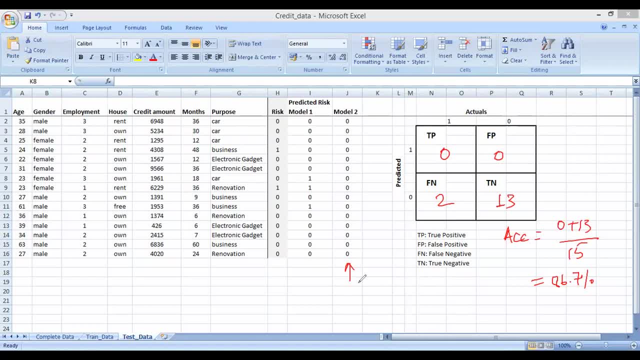 evaluation metric, isn't it? which means my accuracy is somewhere flawed. and this is where exactly accuracy as an evaluation metric fails miserably. and where does it fail miserably? it fails miserably in cases of unbalanced data set. since my data set was unbalanced, i had more number of people who were reaping back. 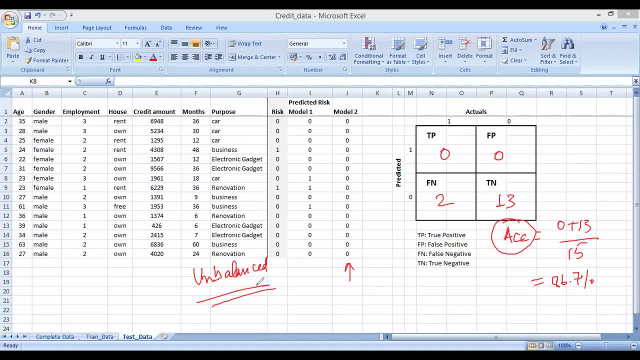 so i thought let's tag or annotate or predict. everyone is a non-defaulter, due to which my accuracy bumped up, but that very small proportion of defaulters. i left them out alone and i left them to loot my bank. so let's try to fix this by creating some kind of a better metric, because, of course, accuracy 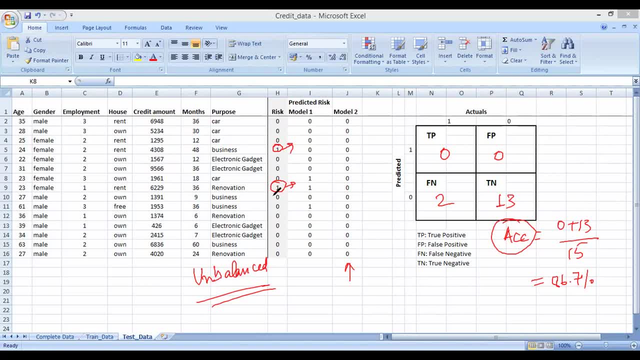 seems to be incapable of capturing the situation. now, this is where i want to introduce the next evaluation metric, which is recall. so recall helps us in this scenario as an evaluation metric. now, if we carefully see what our intent was okay in this kind of a business scenario. my intent was to build a model. 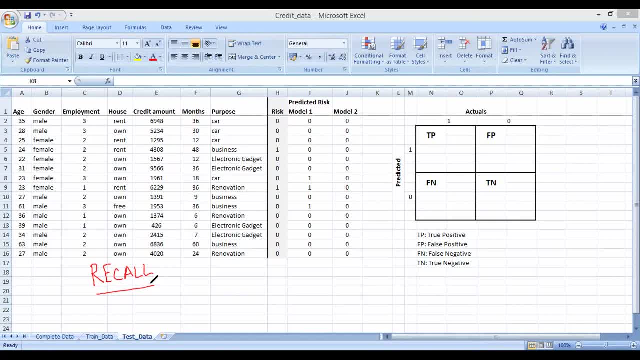 which is able to identify or predict all the details that are important to me, and my goal is to be able to- Or, if I just talk at the data level, I wanted to identify all these ones very, very accurately, Which essentially means that I want to maximize the count of TPs as compared to the count of FN. 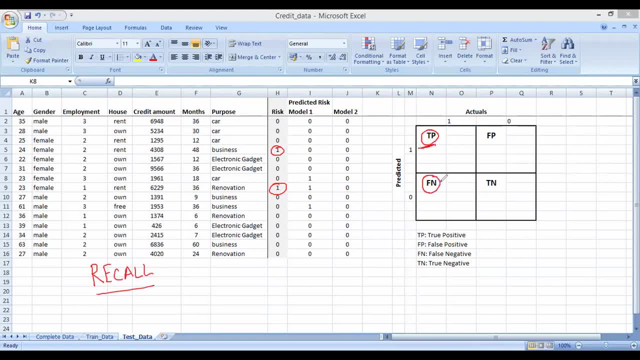 So I want to maximize the true positives as compared to false negatives. This is the basic business logic which I want to follow. Now, if I just try to convert this into mathematics, essentially I want my TP to be as high as possible. 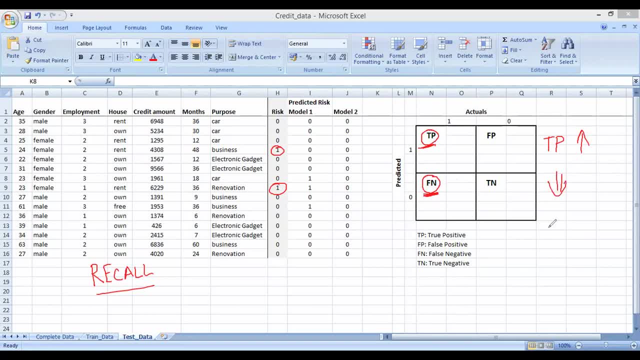 Now, if I put it in a percentage perspective, I want this number of TP over TP+ FN. I want to maximize this proportion And this, this ratio. what you see over here is nothing but my recall. This is that metric. 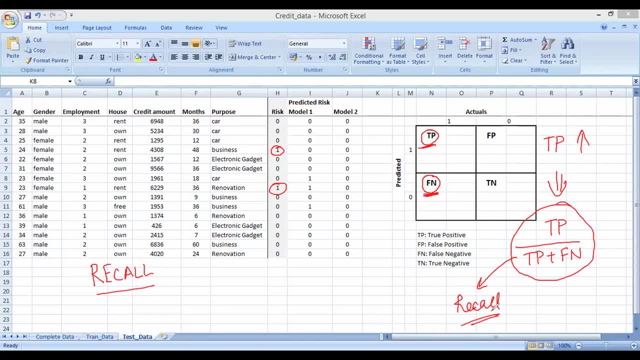 So recall, if I just want to make it a simple English In English English language, if I want to put it, this is nothing but out of total positives, how many could be identified by the model? So this is the question which recall is answering to me. 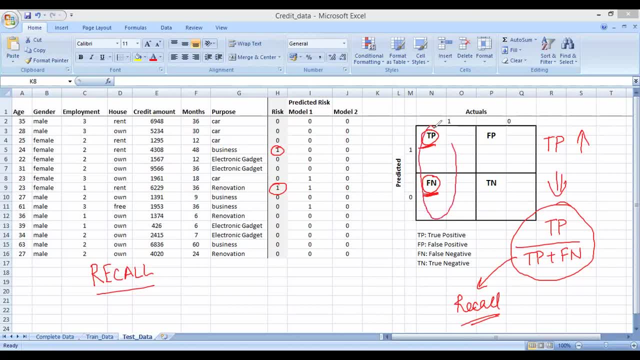 So, out of these total positives which actually exist in the data, how many of them were correctly identified by my model, TP over TP plus FN? So now, if you look at that confusion matrix we were just seeing a little while ago, 00213, if I see the accuracy, it was 13 over 15.. 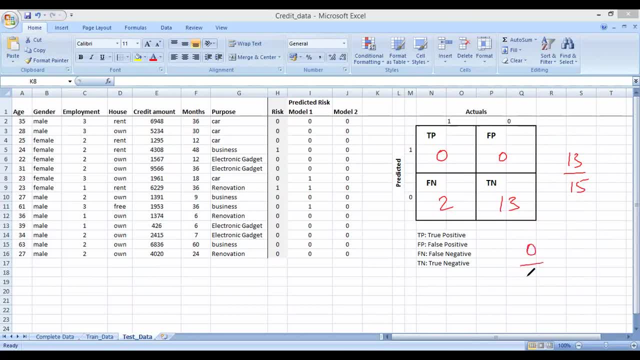 But if I see the recall, it is 0 over 2.. It is absolutely abysmal: 0%. So I fail miserably on recall value and thereby my model is not doing a good job. so I simply strike off model two. 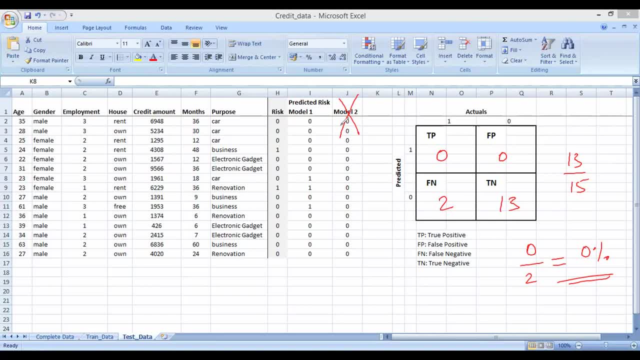 Now I have a different strategy. Okay, me being absolutely lazy. Okay, me being absolutely lazy And a beard fellow, I have a new dirty trick in my mind. Okay, I want to kind of fool the system with this new trick without doing much of work. 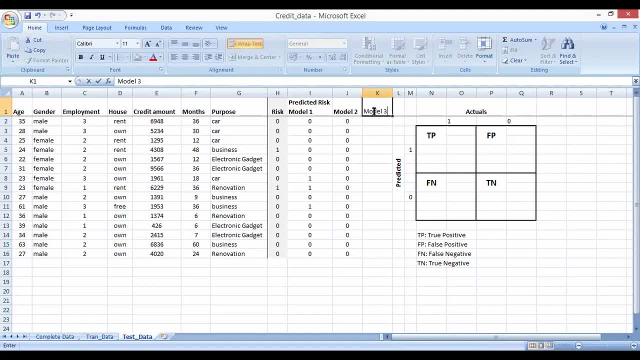 So I'll make another model. I'll make another model, a very simple one, Where I'll say that Let's mark, Let's mark all of them as ones. Let's say: all of them are defaulters. Now, business-wise, up front, we know, business-wise, this is absolutely weird. 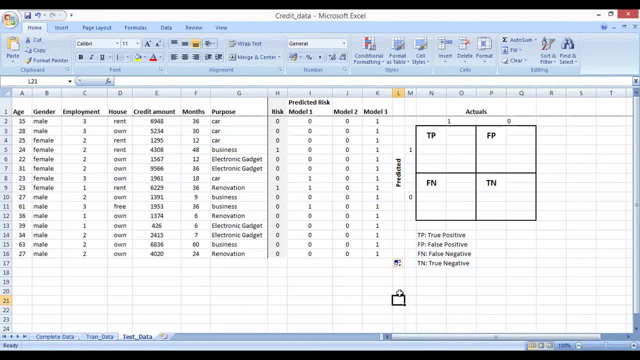 We cannot mark everyone as defaulter. This is a huge loss to the business because if we are marking everyone as defaulter, we cannot give them the loans And thereby we ignore a lot of revenue for us. So this could be a huge opportunity which we have missed to identify because we are targeting all of them as defaulters. 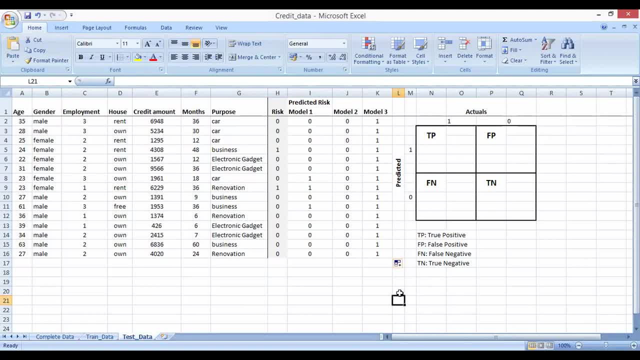 And this is all because of my improper modeling. But let's say I do this And with this let's try to enter the numbers in my confusion matrix. So my TP would be 2.. Just do a quick math or a quick recall of your confusion matrix and you'll identify why I'm entering these values. 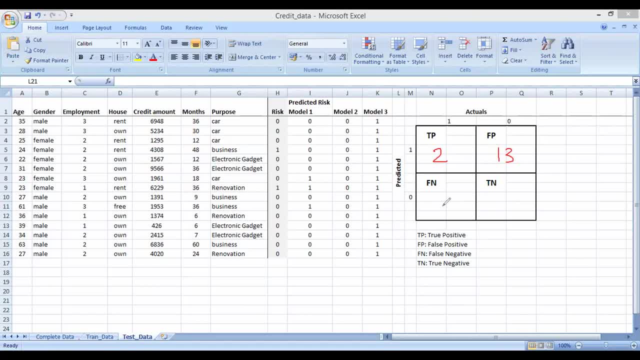 So my TP would be 2,, FP would be 13,, false negative would be 0, and true negatives would be 0. And now if, If I see my accuracy, it would be 2 over 15.. If I see my recall, which we just developed a little while ago, 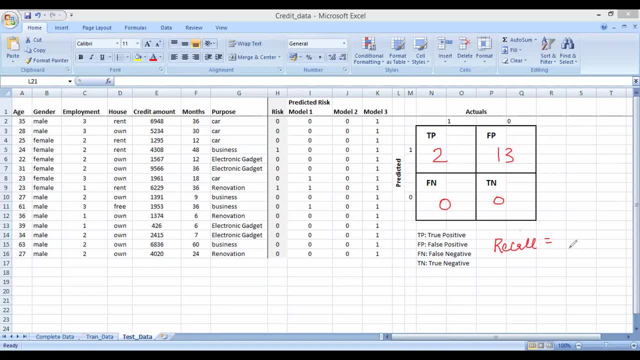 if I see my recall, it would be TP over TP plus FN would be 2 over 2. 1. Wow, 100%, Absolutely phenomenal, Well, isn't it? We did a great, great job, But again, business-wise, we are giving a very, very weird logic. 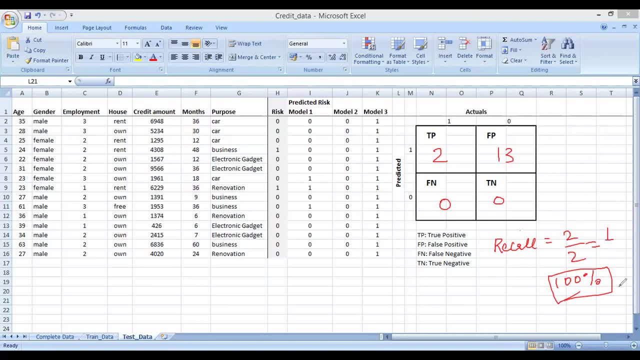 So now we need to refine further and we need to identify more ways to fix this. Now, with this, with this new model- Model 3, I already know that recall alone cannot work well in case of an unbalanced data set. 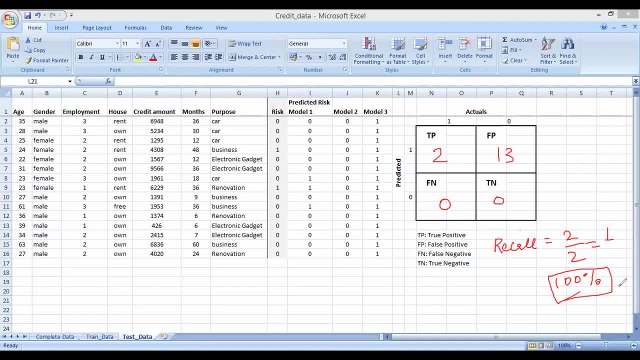 I need to have another metric. I need to have another metric which kind of helps me resolve this problem. And this metric is nothing but precision. And what precision says is: precision says that out of the total identified true positives by the model, how many are actually true positives? 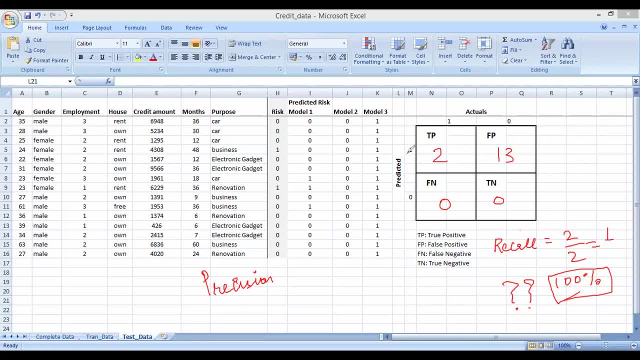 Which means, out of all the all these predicted true positives, out of all these predictive true positives, how many are actually true positives? So if I write this equation, this goes on to tell me true positives over true positive plus FP, And plugging in the values I get. 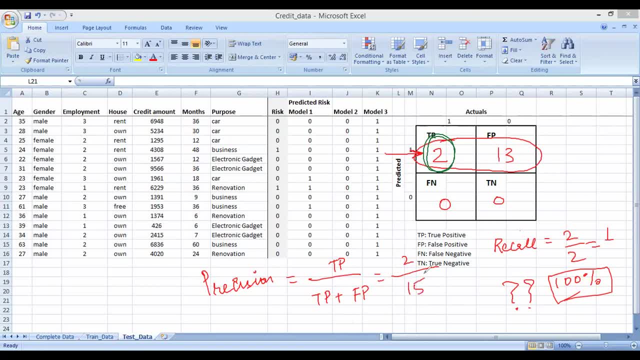 2 over 15, which is nothing but Okonkwo fatigue. 13% is absolutely low, A very, very bad indicator for my model. Now, if I need to summarize, what I get is that my model two failed because of low recall and my model. 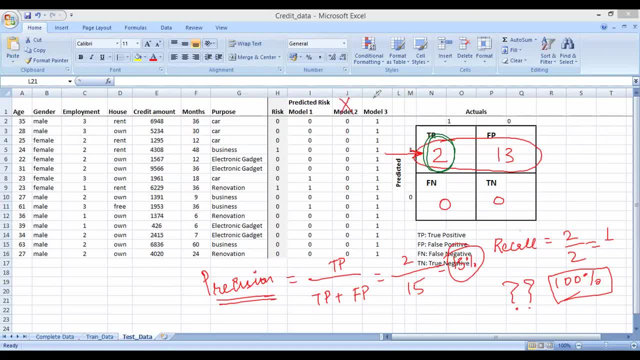 two failed because of low recall and my model three failed because of precision. so, essentially, if I want to fix a good evaluation metric in case of an unbalanced data set, it turns out that I need to do a proper trade-off between recall and precision, which means out of